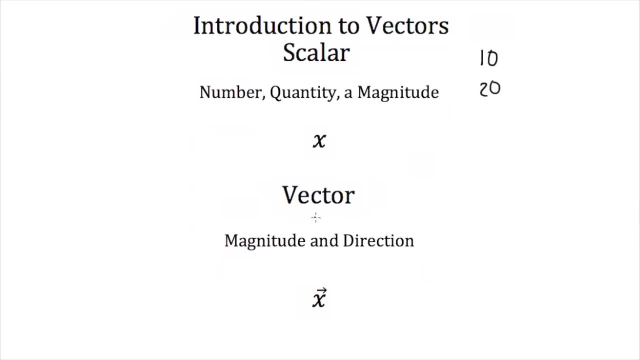 scalars. now we're going to start talking about vectors. Vectors have a magnitude, just like a scalar, but that magnitude is in some direction. So instead of going 20 miles per hour, if I said we were going 20,. 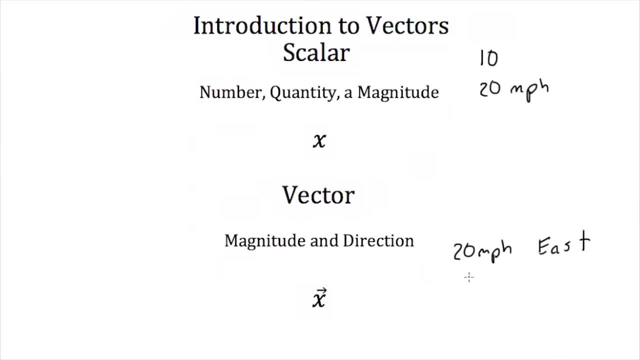 miles per hour east. this is a vector because it has a magnitude, our speed and a direction. We're going 20 miles an hour to the east. Now, whenever you see a vector, it's usually got this little arrow above it. That indicates that what we have here, this variable x, is a vector. Now, 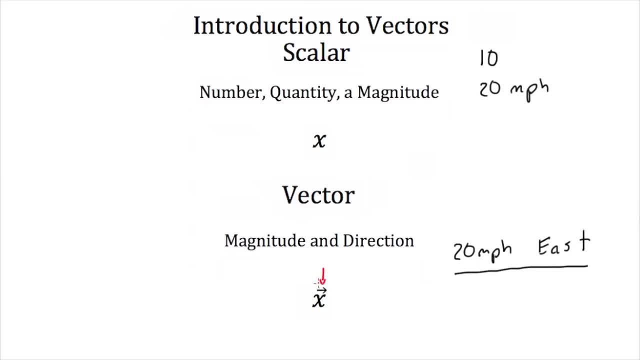 sometimes people will forget to put that little arrow above your variable. So if you're talking about vectors, sometimes they won't have this little arrow above them, but it is correct to put it on top of a variable that's representing a vector. Now, when we graph a vector, 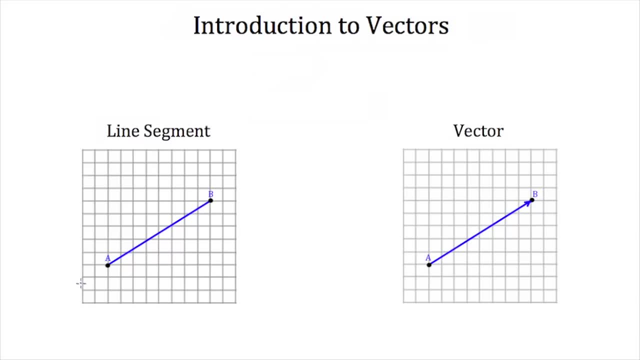 it looks an awful lot like a line segment If I had the line that passes through points A and B. the segment between A and B is my line segment AB. Well, if I said that I was traveling from A to B, then I would have the vector AB. The point A is considered the tail end. 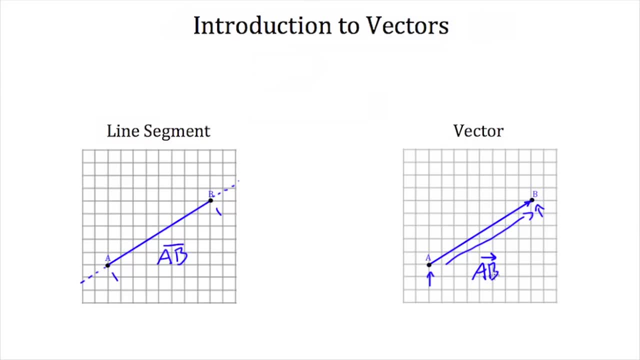 of our vector and point B is considered the tip of our vector And this vector represents us traveling from A to B. The magnitude of the vector is the length of this arrow And the direction is the direction that it's traveling in, which you can represent as a change in y and x coordinates, or you can 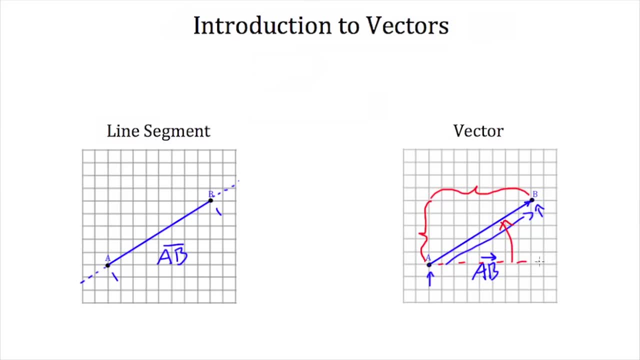 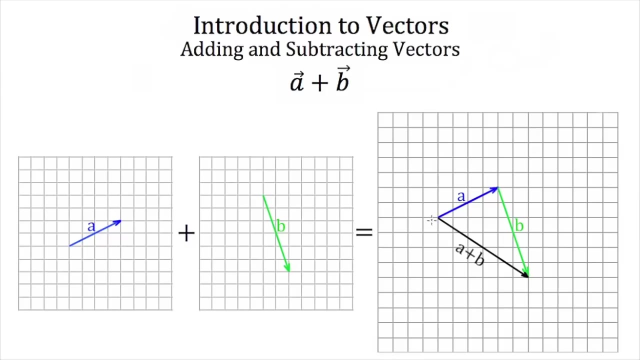 represent as an angle off the x-axis. Just remember that vectors have a magnitude, which is the length of the arrow, and a direction, which is the direction the arrow is pointing in. So now let's talk about adding and subtracting vectors. If we want to add two vectors, all you do. 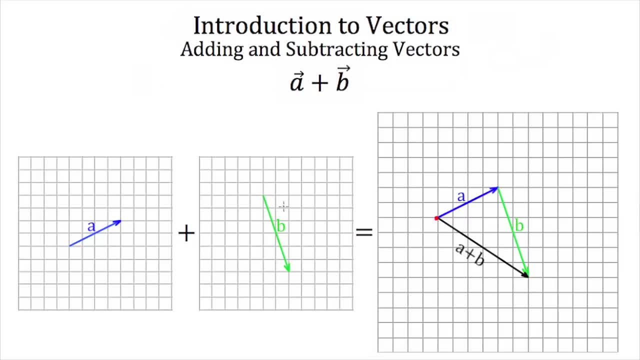 is put them tip to tail. If you have a starting point and we want to add vector A to vector B, we take the vector A and we draw it the same length and in the same direction that it always goes, And at the final point of A. 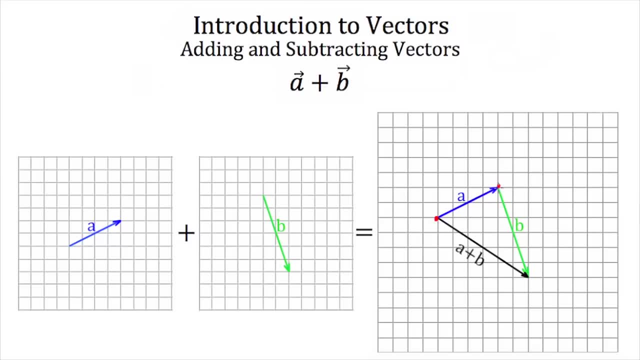 at the end of the vector we draw it the same length and in the same direction that it always goes. And at the tip of A we put the tail of the next vector we're adding. So we put the tail of vector B. Then we draw vector B at the same length and the same direction that B always goes. 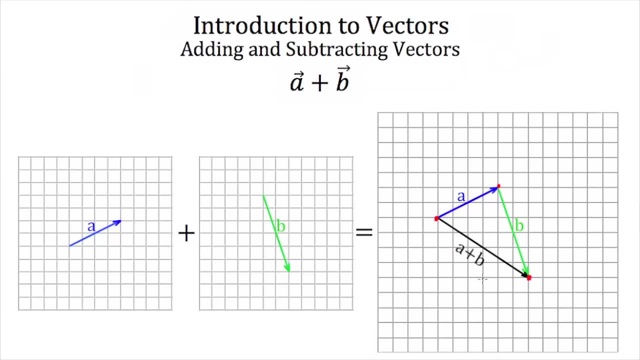 in And at the tip of B we will find the tip of the vector AB. The vector AB starts at our original point and travels to the tip of B as long as B is tip to tail with vector A. So when we add two vectors, we usually make this kind of a triangle, And whenever you want to add, 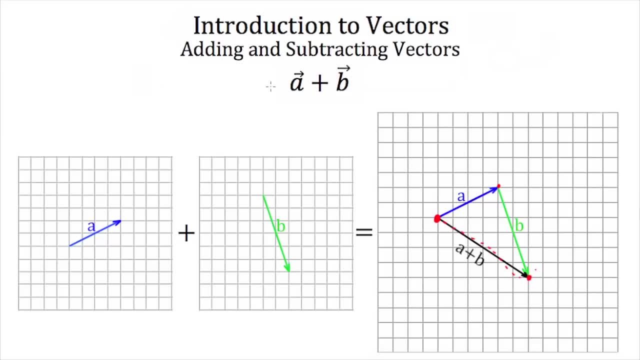 vectors. you just keep putting them tip to tail. It's also important to notice that it doesn't matter what order we add our vectors, Just like adding numbers. If you were to add 3 to 4, you would get the same number as if you added 4 to 3.. Well, if you add vector A, 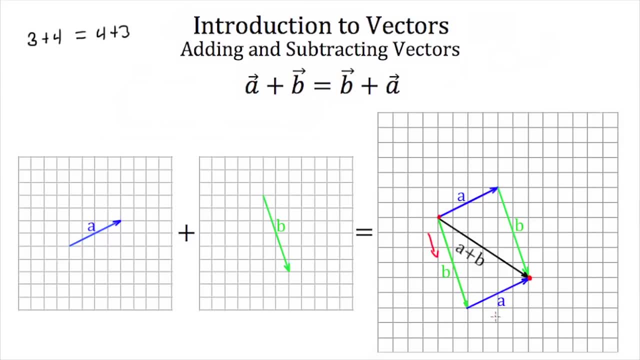 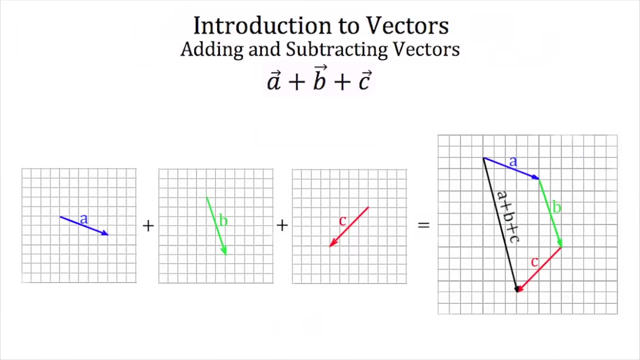 to vector B, you will end up at the same point as if you add vector B to vector A. So again, it doesn't matter in what order you add vectors, The sum is always the same. Now let's say we wanted to add more than two vectors together. Say we wanted to add three. 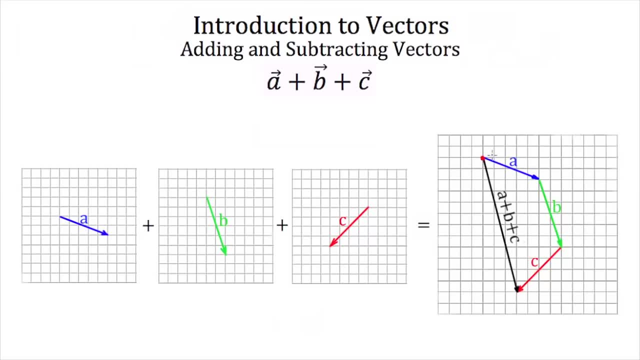 or four vectors. Well, the steps are exactly the same. You draw A at some starting point in its length and direction, And then, at its tip, you put the tail end of B. And you draw B at the same length, in the same direction. At the tip of B you put the tail end of C And at the tip of C 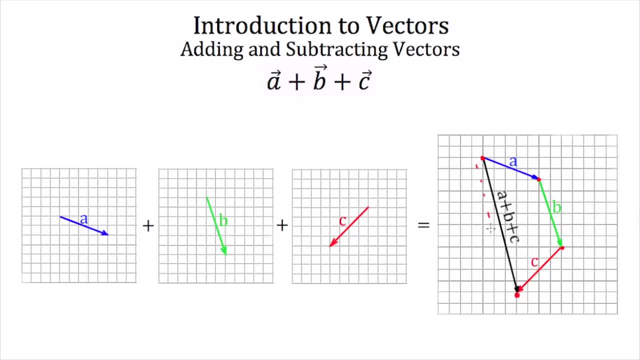 is the location where the vector A plus B plus C will end up. So if you're adding more than two vectors, if you're adding three or four or five, just put all the vectors together, Tip to tail and wherever they end up is where the vector of your addition will end up. 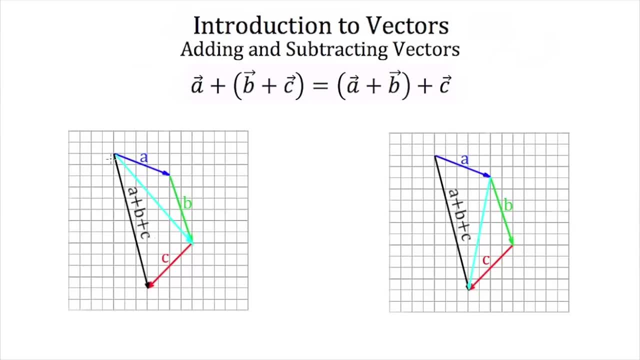 Now again, even if you're adding more than two vectors, it doesn't matter in what order you add them together. If I were to add A to B, I would end up here. Then, when I add C, I end up at the. 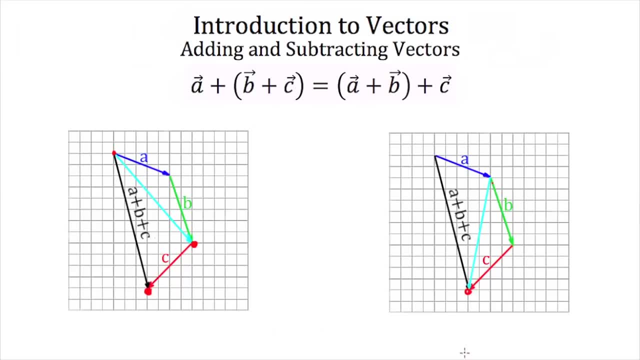 same place as if I added B and C together. So if I were to add A to B, I would end up here. Then, when I add C, I end up at the same place as if I added B and C together together and added that to A. So it doesn't matter in what order you add. 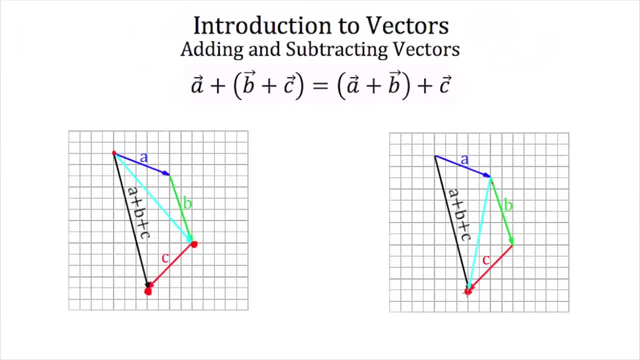 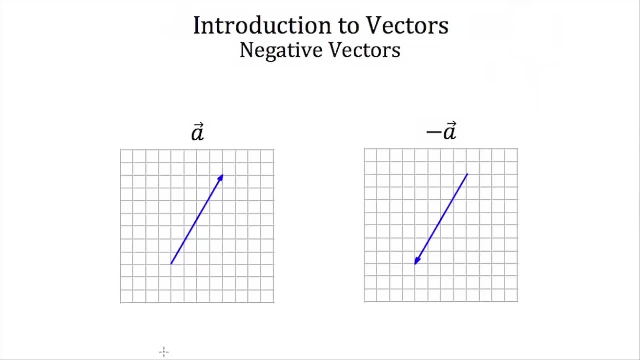 vectors. you should always end up at the same place. Now, typically we do not subtract vectors, We add a negative vector. A negative vector is the exact same vector as the positive version, except it goes in the opposite direction. So if vector A here is moving up and to the right and it is, say, five long, then 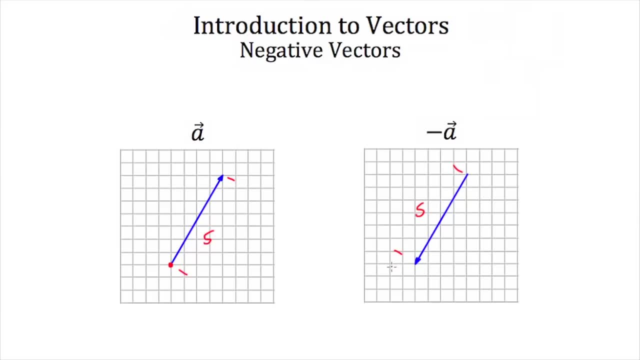 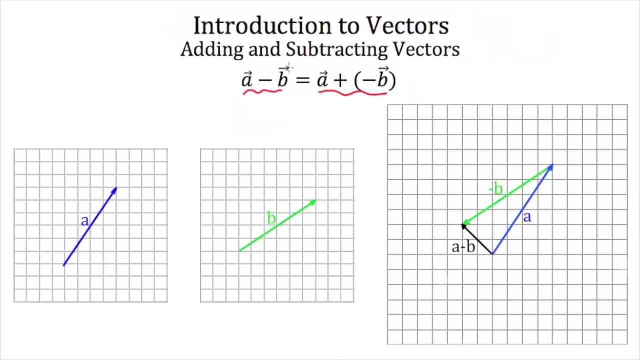 negative A is also five long and moves in the exact opposite direction. This vector moves in a downward and leftward direction. So the magnitudes are the same for a vector and it's negative, but the negative vector just moves in the opposite direction, moves in the opposite direction. So if you wanted to subtract vectors instead, 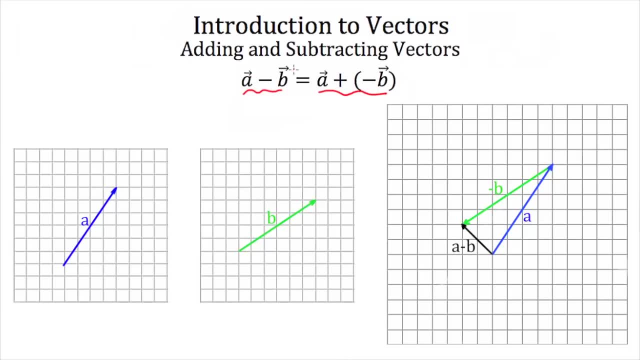 you would add the negative of whatever vector you're subtracting. So if I wanted to subtract B from A, I would instead add the negative of B to A. So here I have vector A and here I have vector B, and if I want to subtract them, I draw A like. 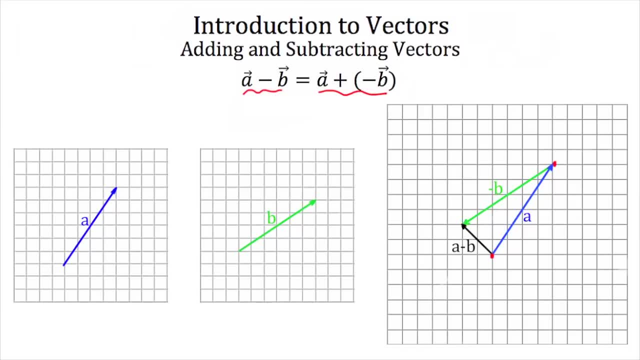 I normally would, And then, at the tip of A, I instead put the negative of B. Realize that B usually goes in this direction, but since it's negative, it's going to go in the opposite direction, the same distance, until we get to this. 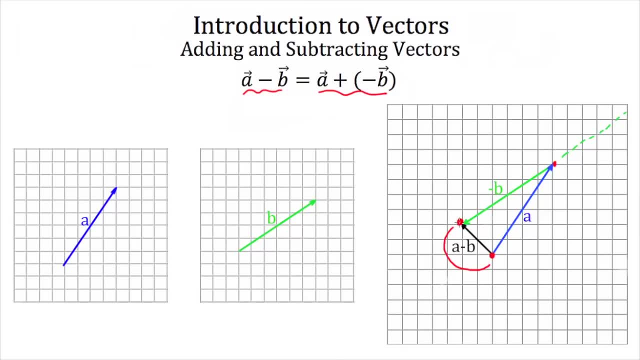 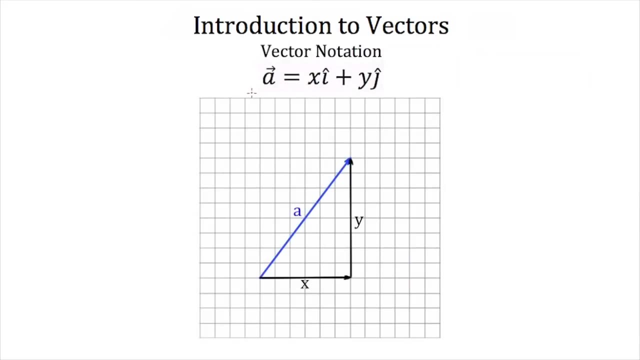 point. And then this vector. here is the vector A minus B. From the tail end of A to the tip of A, I draw B. So that's how you subtract vectors. So now let's talk about vector notation. Here we have the standard formula for. 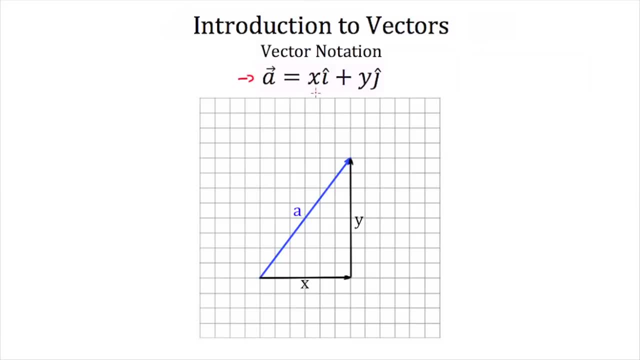 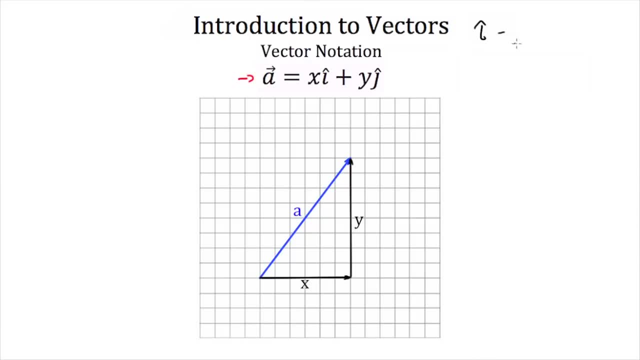 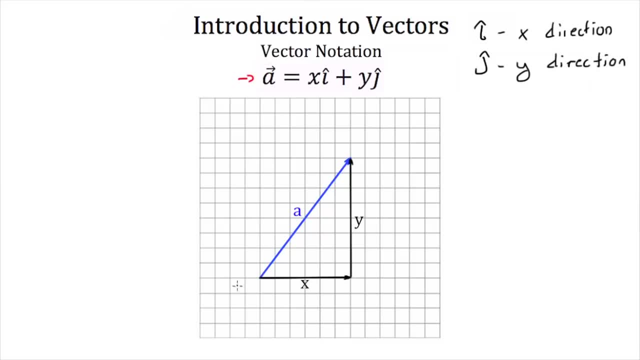 move in the Y direction. move in the Y direction. So if we wanted to write vector A in standard notation or vector notation, we need to know the amount we move in the X direction. Well, this guy is moving in the X direction and it's moving 8 in the Y direction. So we would say that 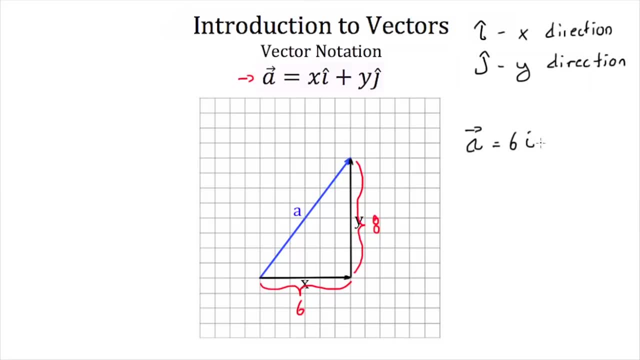 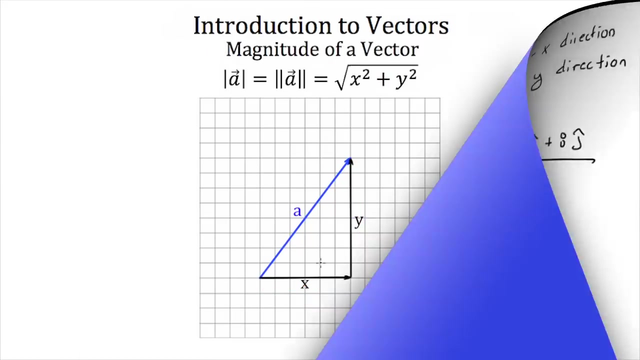 vector A, that's equal to 6 i-hat plus 8 j-hat. Now don't worry about these i's and the j's, that just indicates the direction: 6 in the X, 8 in the Y. So this is vector A written in vector notation: 6i plus 8j. 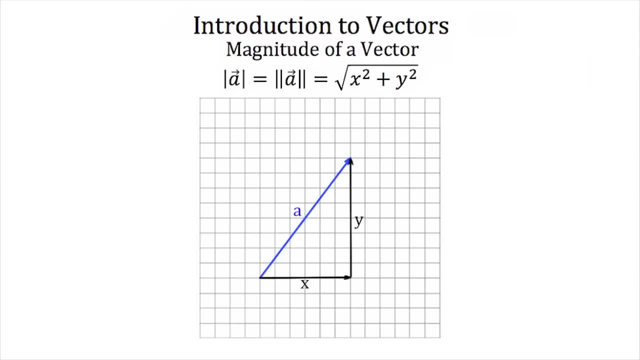 Now we use vector notation because it makes it easy to algebraically add vectors. It also makes it easy to find the magnitude of a vector. Remember vector A here in standard form is 6i plus 8j-hat. If I want to find the magnitude of my 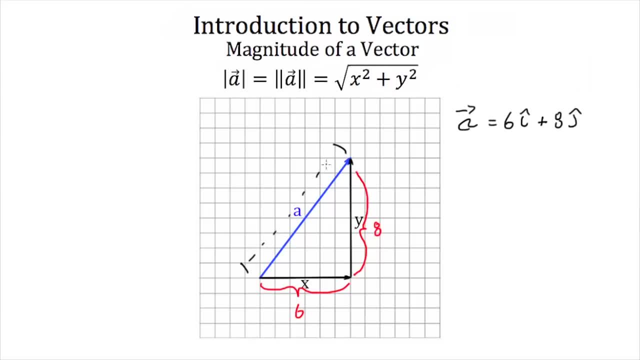 vector which, remember, is the length of my vector. well, the X and Y can be calculated by rotating the vector y- z-hat. So I can write this vector A minus the Y- z-hat, I put a negative up to the x-hat and then I put in a negative probably. 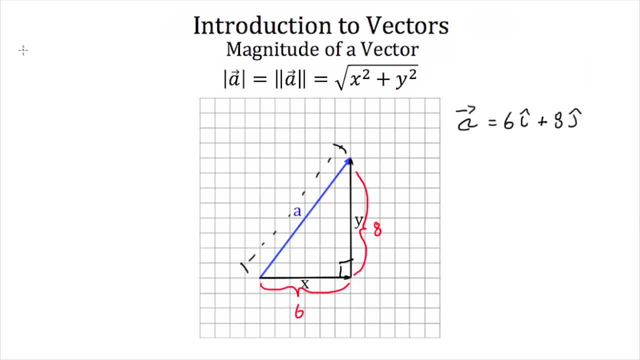 negative value on both sides. Then when I move back, I create a 90 degree angle here, which makes this the hypotenuse of a right triangle, Which means you can use the Pythagorean theorem, which would tell us that our hypotenuse, squared, would be. 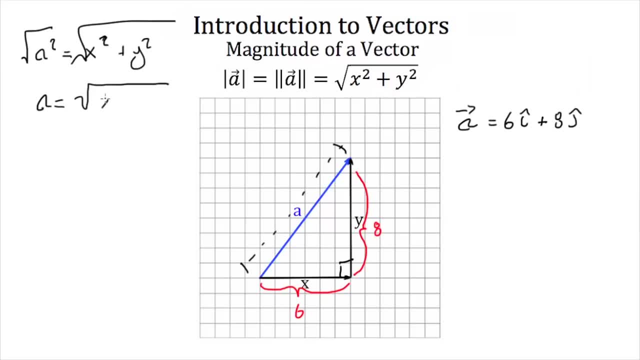 equal to the square root of x squared plus y squared. Typically, when somebody's asking for the magnitude of a vector, they will put the vector in absolute value or in this double absolute value sign. So if you ever see a vector in an absolute value sign or a double absolute value sign, 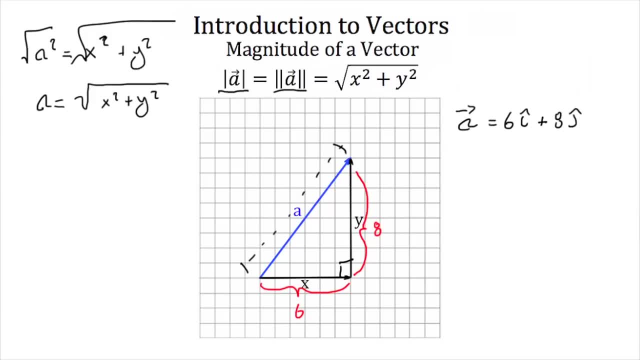 that means they're looking for the magnitude of that vector, and you can use this formula to find the magnitude of that vector. Here our x is 6 and our y is 8.. If you plug that in, you'll have 6 squared plus 8 squared underneath the square root, or you can. 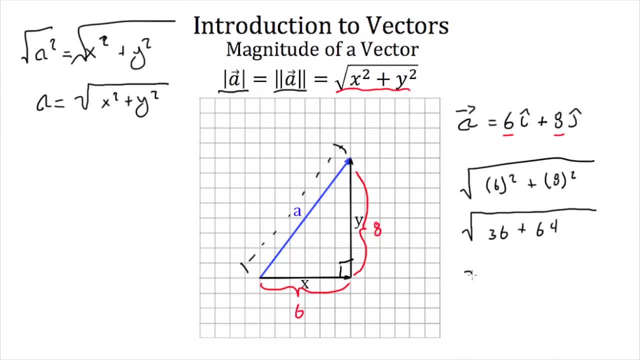 say the square root of 36 plus 64.. Or you can say the square root of 100, and that's equal to 10.. So the magnitude of a is equal to 10.. Now, like I said before, vector notation can help us add and subtract vectors. 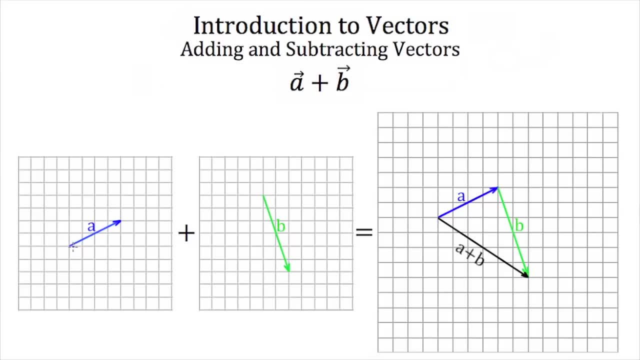 Here I have vector a. Vector a is moving 4 in the x And 2 in the y. I also have vector b. Vector b moves 2 in the x And it moves downward or negative 6 in the y. So if I say vector a is equal to 4, i hat plus 2, j hat. 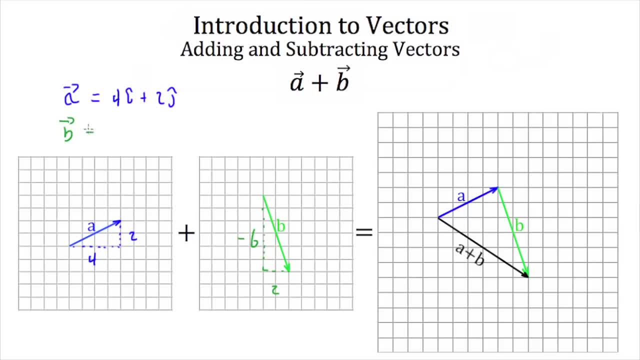 And then vector b, That's equal to 2. i hat plus negative 6 j hat. When I want to add these vectors, I can add just the x's and just the y's. So a plus b should have 4 plus 2, a movement of 6 i. 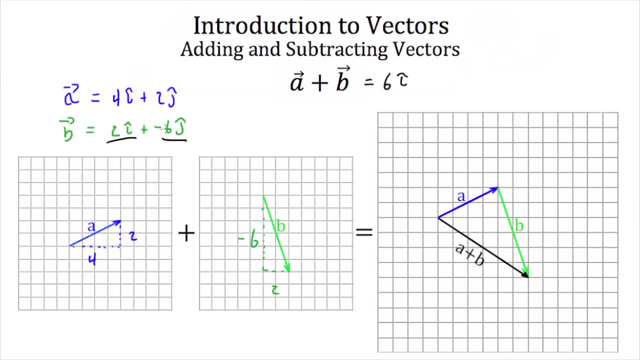 And then 2 minus 6 would be minus 4j. Well, here we have our addition. graphically, This guy is moving in a negative: 4 in the y And 6 in the x. 6 in the x, Negative, 4 in the y. 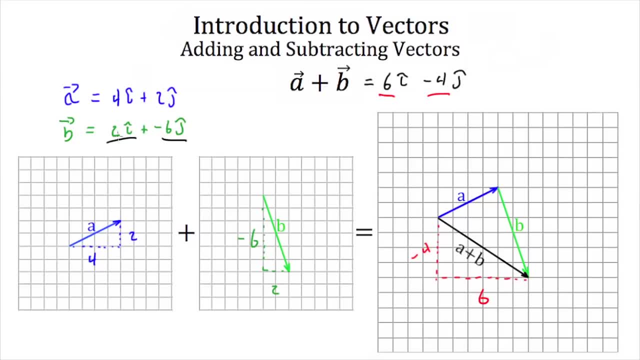 So by writing your vectors in vector notation you make it easy to add and subtract vectors, Because you just add The x's or the i hat terms And then you just add the y's or the j hat terms. Now, often times you'll see a vector being multiplied by a scalar. 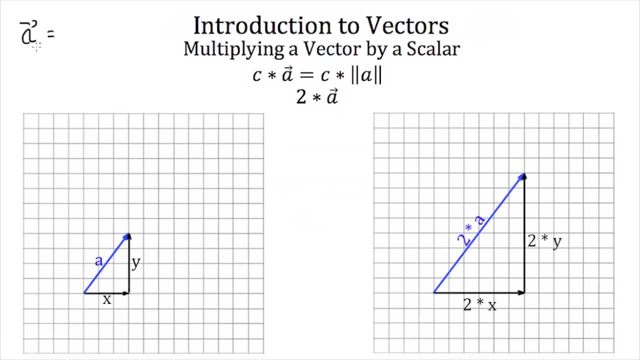 Say A was the fact that we were going 20 miles per hour To the northeast And somebody said we were going to Double our speed. So we were going to take our vector a And we were going to double it. 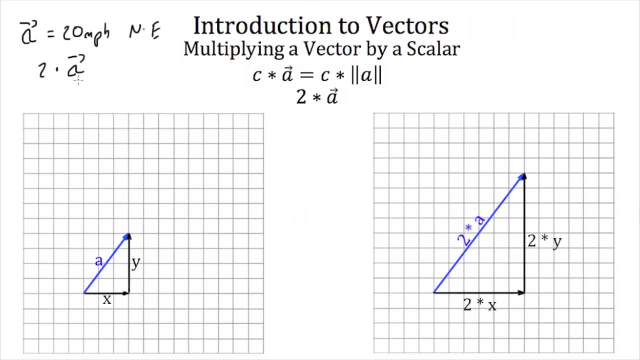 Multiply it by 2.. Well, if we're doubling Our vector, that means we're going to be going 40 miles per hour To the northeast. So when you multiply A vector by a scalar, That's the same As basically just. 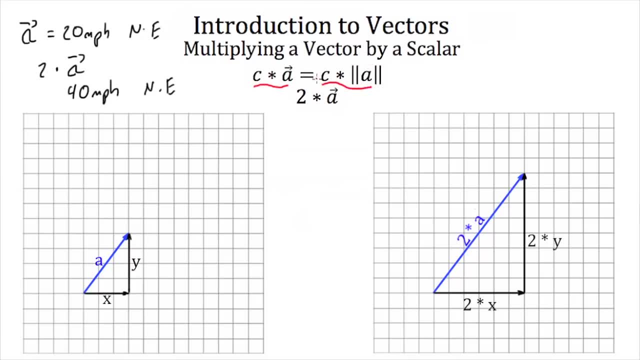 Multiplying the magnitude Of that vector by the scalar. The scalar does not change the direction. So if I have vector a here, It has an x value of 3. And a y value of 4. So I can say A is equal to. 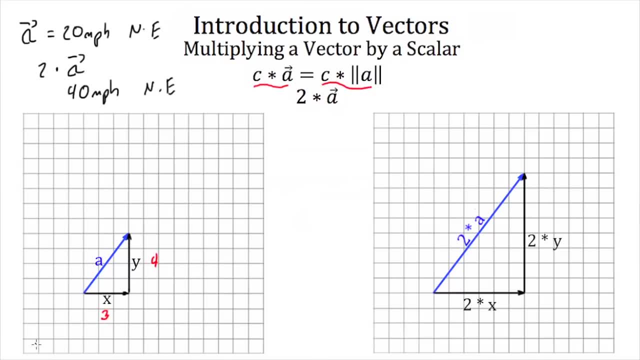 3 i hat, Plus 4 j hat, And I wanted to multiply this by 2.. Well, my magnitude is multiplied by 2.. So I can say A is equal to 3 i hat, plus 4 j hat, And I wanted to multiply this by 2.. 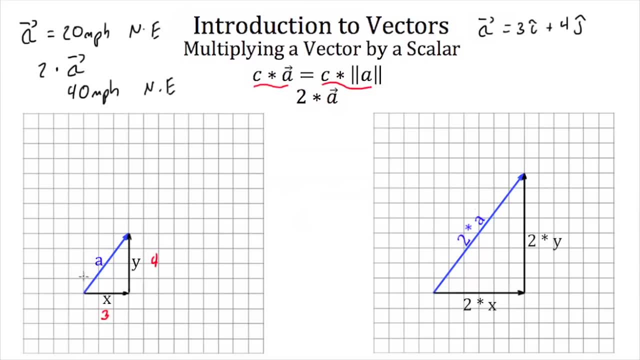 Well, my magnitude is multiplied by 2. Which means the length of my vector Is now twice as long. Well, if one of my vectors Goes 3 in the x and 4 in the y, Then two of my vectors In the same direction. 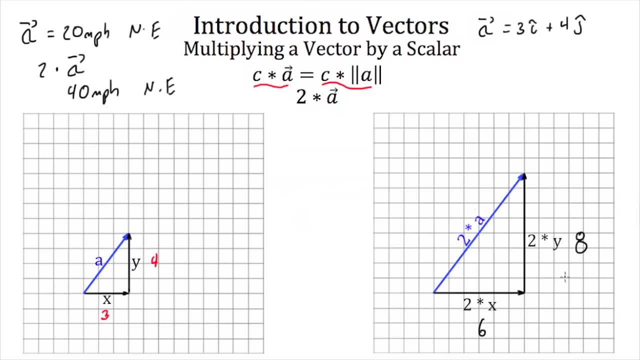 Will go 6 in the x And 8 in the y. So when you multiply A vector by a scalar, You can either multiply the magnitude By that scalar Or you can multiply Both the x component And the y component. 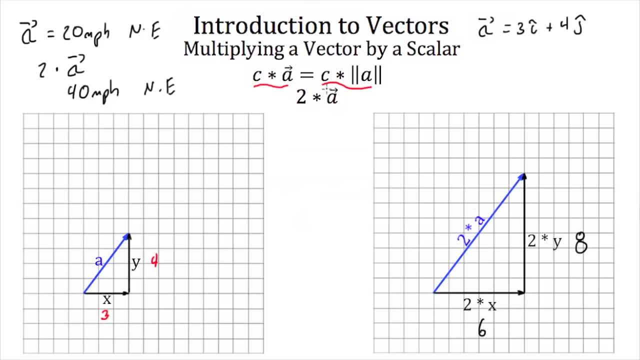 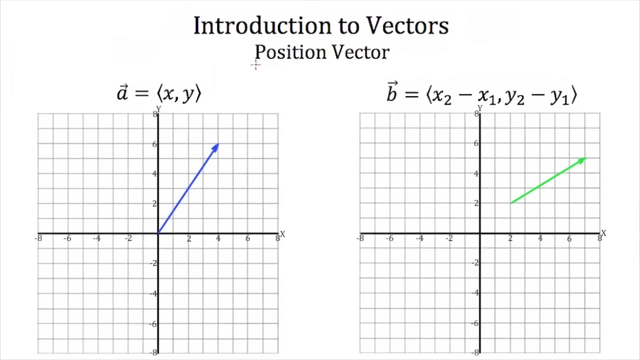 So 2 times the vector A Would get us 6 i hat Plus 8 j hat. So that's how you multiply A vector by a scalar. Now, lots of times When we talk about vectors, You'll hear the term. 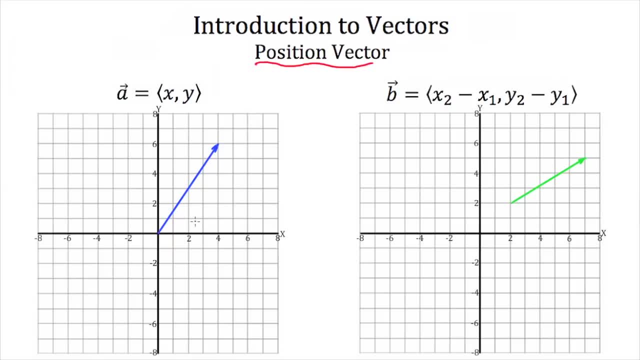 Position vector. Position vectors are just vectors Where the tail of them Starts at the origin, And sometimes they're written like this: Here we have Vector a. It moves 4 in the x And 6 in the y. 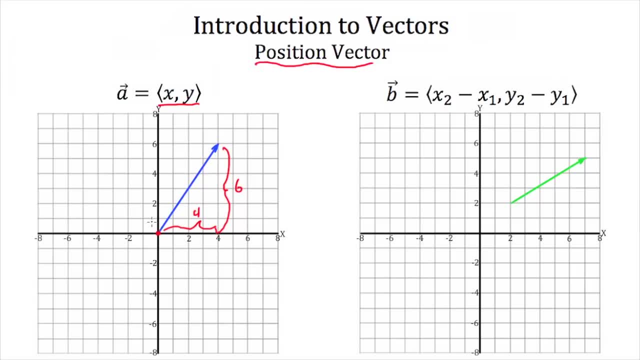 But vectors aren't always At the origin. Sometimes they're floating out here In space, If you wanted to find What we call the equivalent Position vector, Where, if we move this same vector Down here, So the tail was at the origin. 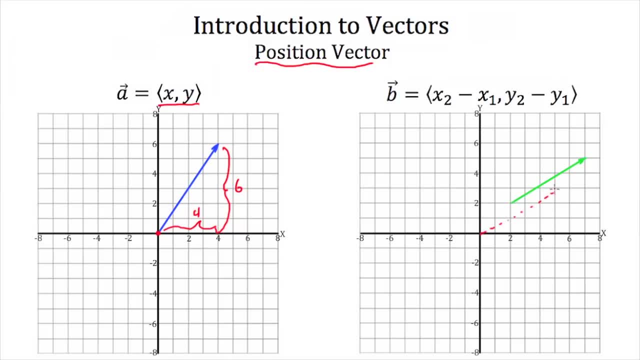 Then we would end up With the same vector. It would just be moved down here. So the tail Is at the origin, And if you wanted to find The equation of that vector, Then you just take it's starting X position. 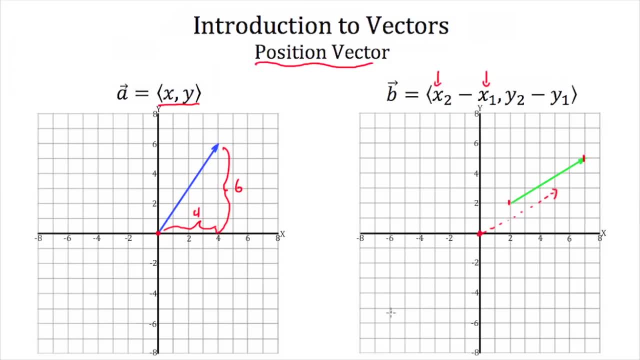 And it's final x position. X1 would be the starting And x2 would be the final. And you do the same thing for the y's: It's starting y position And it's final y position. Starting y position And final y position. 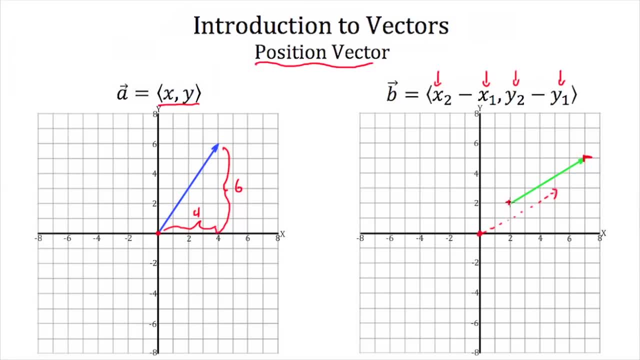 But you can do this With a vector. We start with an x value of 2. And we go to an x value of 7. So b Would be 7 minus 2.. Y would be 2 to 5.. 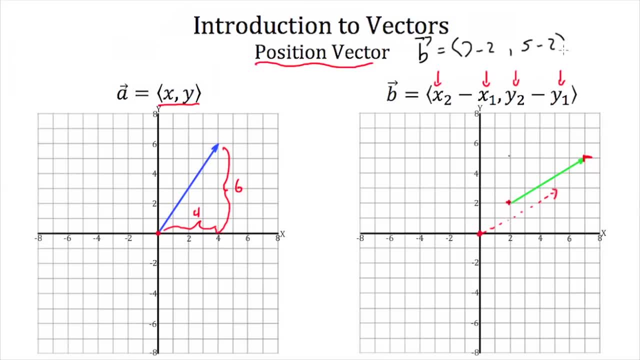 So 5 minus 2. And vector b Would have an equivalent Position: vector Of 5. And vector b Would have an equivalent. You could also write vector B as 5i-hat plus 3j-hat. This vector moves in the. 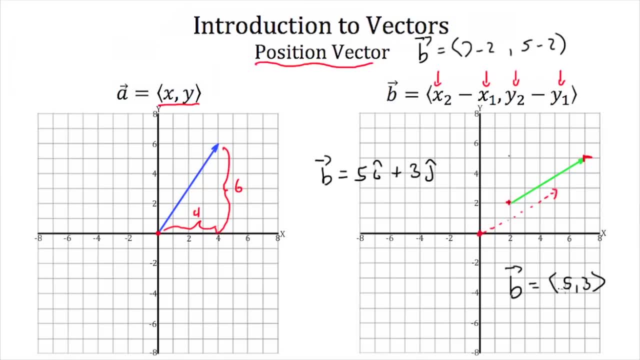 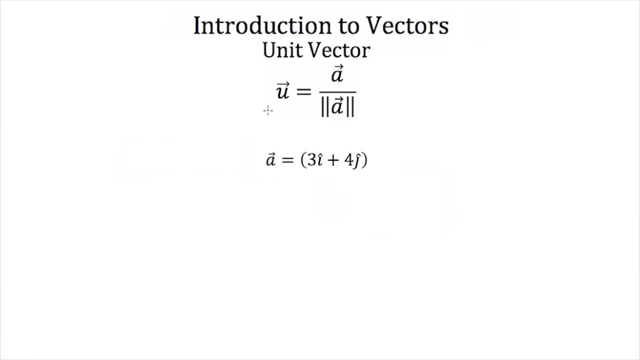 x-direction 5 and in the y-direction 3, regardless of where it's positioned. Now the last thing we have to talk about are unit vectors. Unit vectors are usually indicated by this U with the vector sign over it. Now, if you were trying to find, 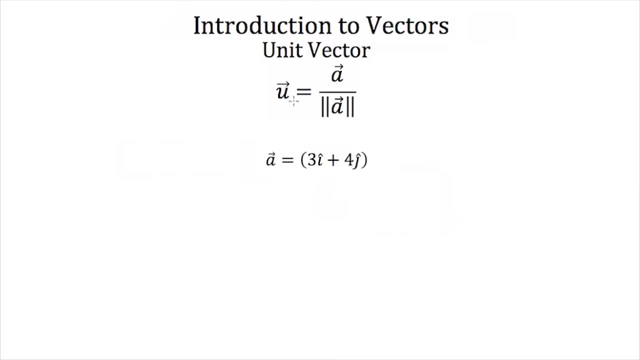 the unit vector of vector A. sometimes you'll see U with this little subscript A. This is the unit vector of vector A. Now, a unit vector is a vector that goes in the same direction as vector A, except it only has a magnitude of 1, or you can think of it as being only one unit long. 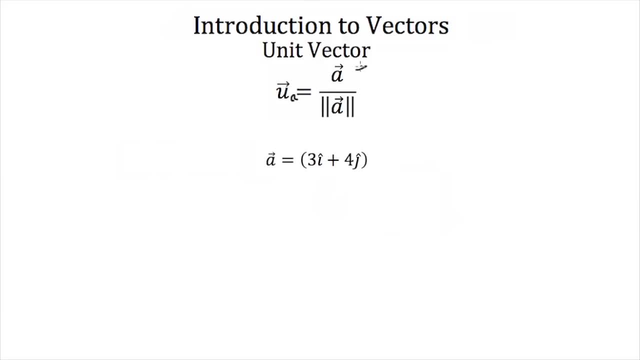 The easiest way to find a unit vector is to take the vector that you have and divide it by the magnitude of your vector. So if I wanted to find the unit vector of this vector A, 3i plus 4j, I would have to find the magnitude of this. 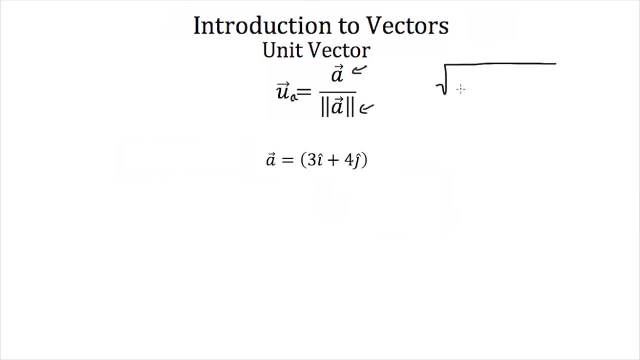 first. Well, the magnitude is just the square root of 3 squared plus 4 squared. This is the square root of 9 plus 16, or you can think of that as a square root of 25, which is equal to 5.. So the magnitude of vector A: 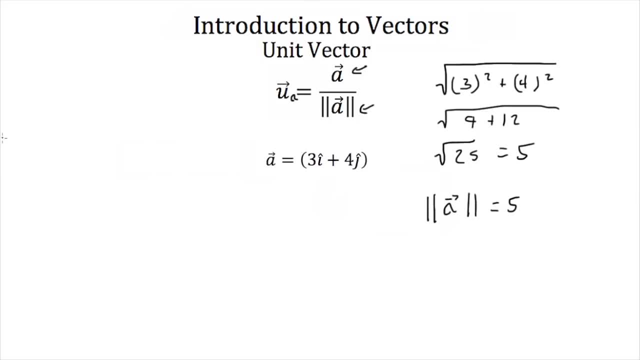 is equal to 5.. If I want to find the unit vector of vector A, I take vector A, which is 3i plus 4j-hat, divided by 3j-hat, my magnitude, which is five. Now this is a fraction.